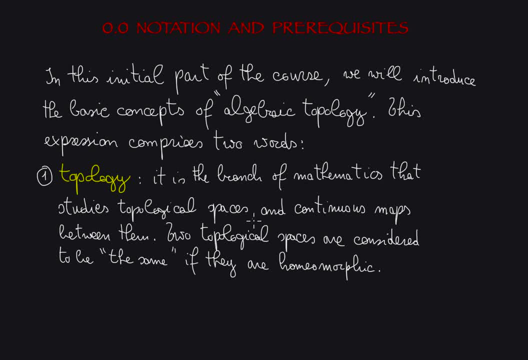 is a branch of mathematics that studies topological spaces and continuous maps between them. Two topological spaces are considered to be the same, in a sense, if they are homeomorphic. Two topological spaces being homeomorphic, I remind you, that means that there are two. 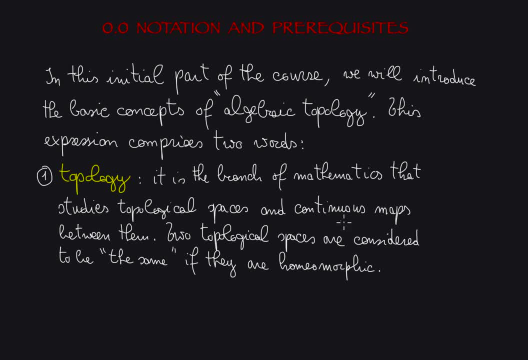 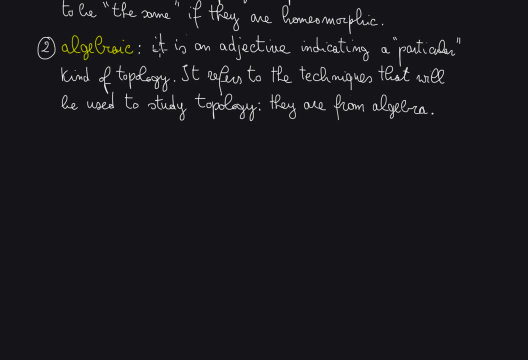 maps going from one space to another and from the codomain of the first map to the domain, in such a way that the composition of these two continuous maps is the identity if taken on the domain and then if taken on the codomain. The second word is algebraic. Algebraic is an adjective indicating a particular kind. 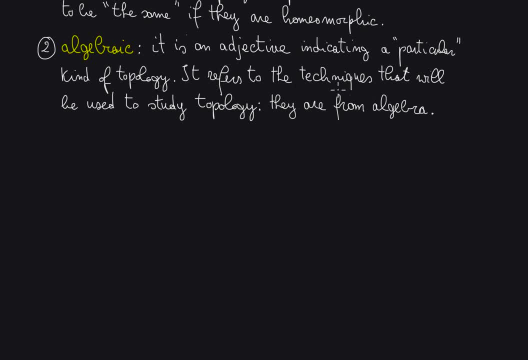 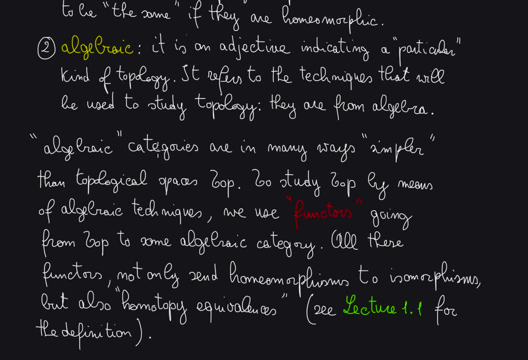 of topology. Specifically, it refers to the techniques that will be used to study topology. These techniques come from algebra. Algebraic categories are in many ways simpler than topological spaces, whose category usually is denoted by top. To study top, which is a very complicated 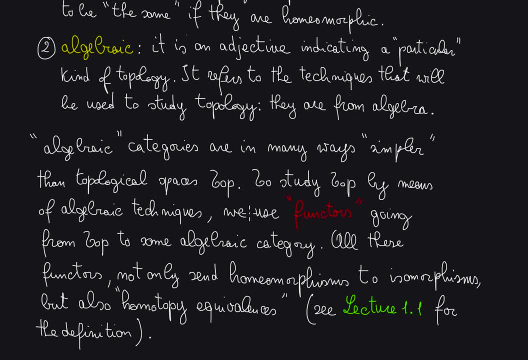 category by means of algebraic techniques. we use functors going from top to some algebraic category. All of these functors not only send homeomorphisms to isomorphisms, but also homotopy equivalences, which is somehow more relaxed concept than homeomorphisms. 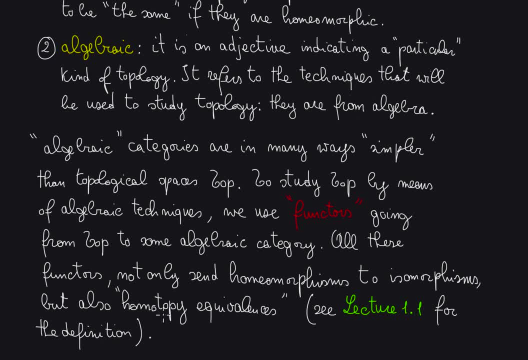 See the next lecture, lecture 1.1, for the definition of homotopy equivalences. Typically algebraic categories will be things like category of groups, category of modules, cassini, ajac and allotty over a ring, a commutative ring or even non commutative rings. the prerequisites: 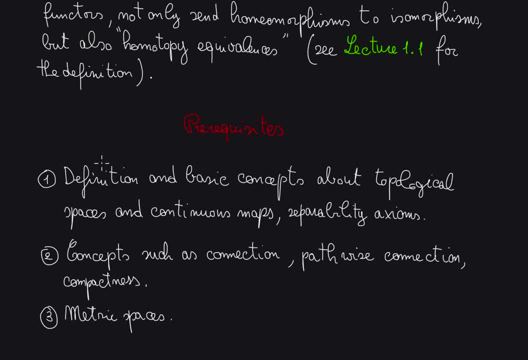 for this course are essentially of these three kind: definition and basic concepts about topological spaces and continuous maps, in particular separability axioms. and then the second group is concepts such as connection, pathwise connection and compactness of topological spaces and third matrix spaces. so one should be